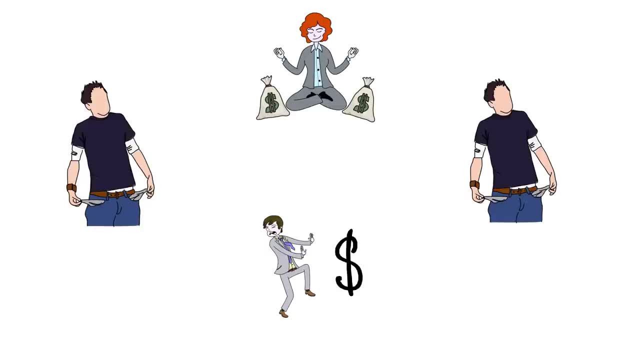 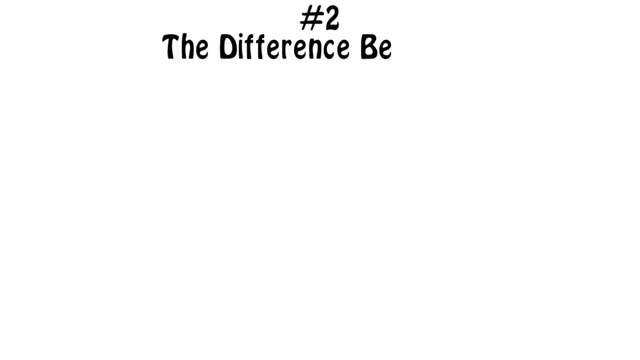 financially-driven society while neglecting their financial life, all because they think of money as not important. Number two: they teach the difference between assets and liabilities. One of the most important and basic concepts of building financial independence is understanding the difference between assets and liabilities. 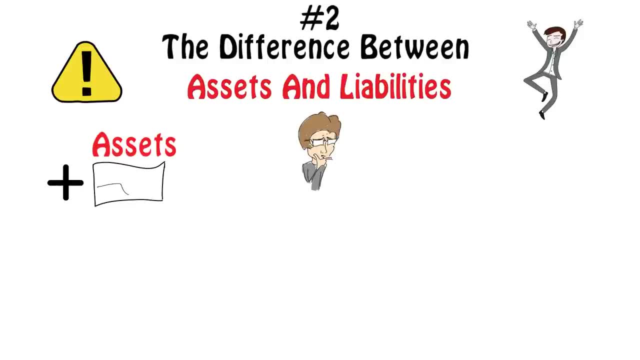 If you haven't heard of these before. assets are like things that bring money into your bank account, And liabilities do the opposite. They take money out of your bank account, For example, a house, and you rent it out to someone. it is an asset because it brings cash flow every. 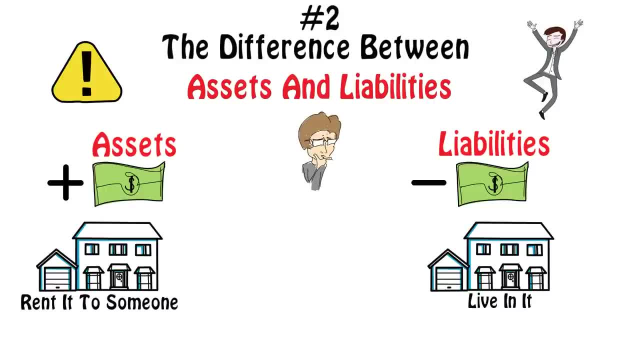 month in form of rent. If you buy a house to live in, then it's a liability because it takes money out of your pocket every month. Many rich parents teach their kids to build and buy assets and avoid liabilities. This way they can create a business or investments. 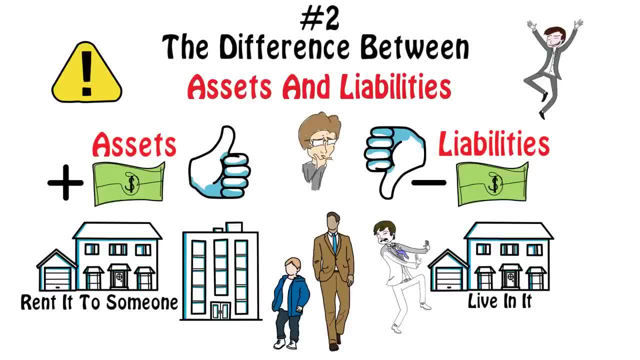 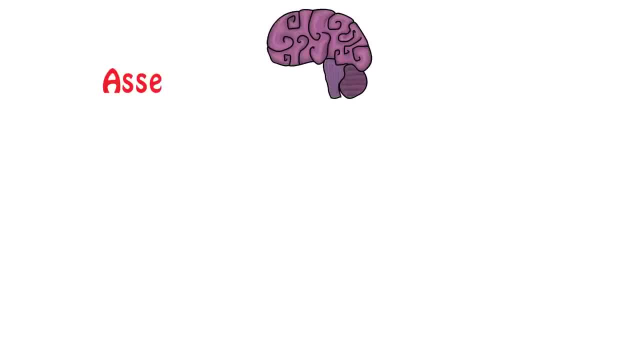 that generate cash flow on a recurring basis and avoid the things that generate a negative cash flow on their bank account, so they can have a surplus of money. They also understand the power of using assets to detach your time from your income, Since assets generate cash. 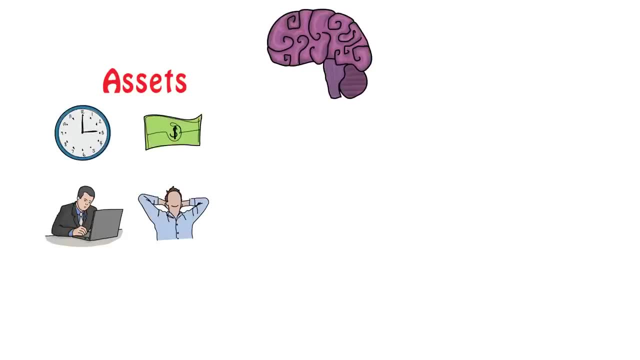 flow. whether you are physically putting in the work or not, you are able to scale and use your time to develop more assets. Rich people often focus on understanding and teaching the spending patterns of the poor versus the rich and why some people earning the same. 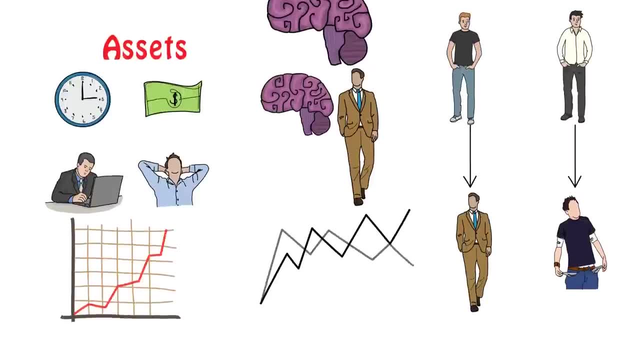 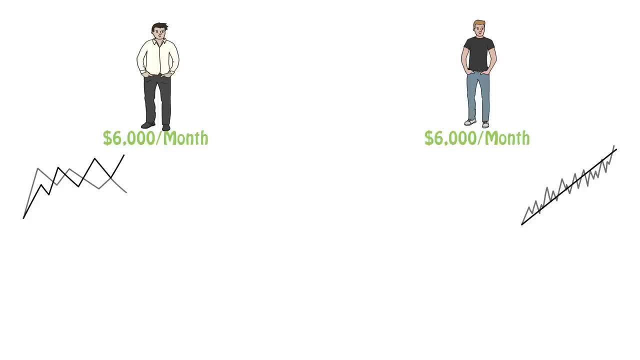 salary end up becoming rich, while others stay poor. For example, let's say that we have two people making $6,000 per month, but they have very different spending patterns. The first one gets their paycheck and pays his bills and enjoys his money going out. 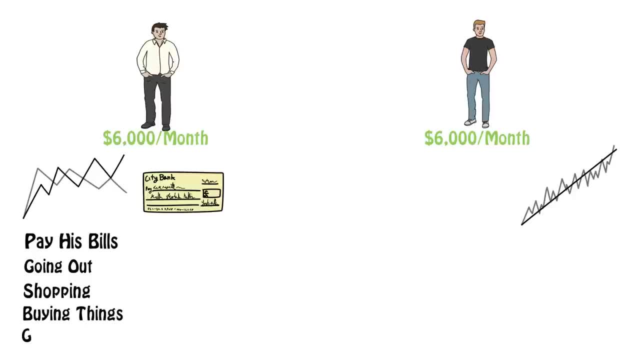 shopping, getting the newest phone and the latest TV, indulging in the finest restaurants, getting a new car, a nice house and all of that nice stuff. They typically spend their money on things that make them look good and wealthy, but they actually come back home. 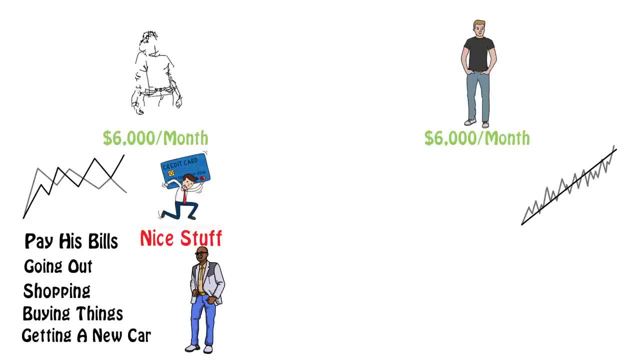 to bills and a lot of debt. They typically have little to no savings and have years of debt on their credit cards, car payments and mortgage payments. They are stuck in. the rat race will take years to get out. Now let's see the second person. 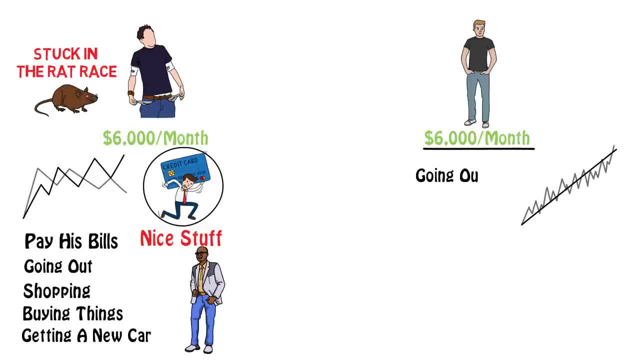 He also makes $6,000 per month. But this person does not buy a nice house or a nice car. He doesn't go out every weekend and he doesn't go to the fancy restaurants. He occasionally buys clothes when he needs them, but he doesn't follow the fashion trends. 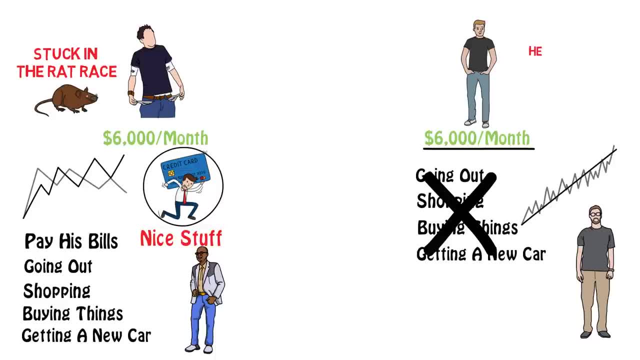 every season. He lives on a $3,000 a month budget and puts away the other $3,000.. By the end of the year he has $36,000 and puts them into cash flow investments. that increases his monthly income. He continues living on his $3,000 a month budget and by the following year he's able. 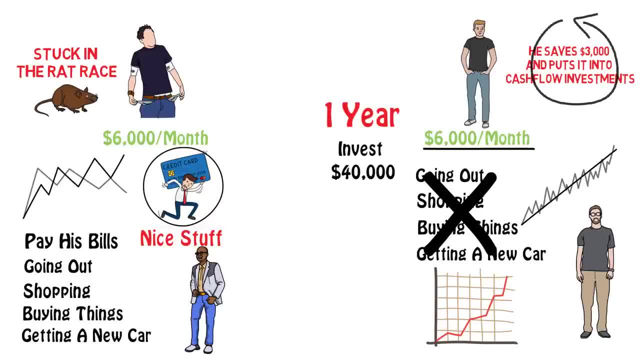 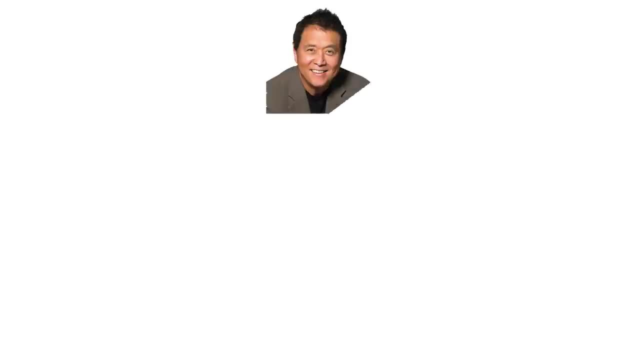 to invest not $36,000 but $40,000, since he increased his income into investments that generate cash flow. Ten years later, these two individuals will be in two completely different places, all due to their spending habits. There's a quote from Robert Kiyosaki that says: looking good but going nowhere. 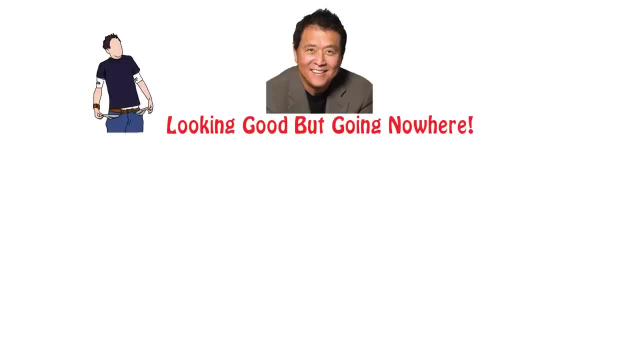 Which means that many people spend their money to look good. They look rich while actually being poor. In the meantime, rich people look poor while getting rich. Now a lot of people might be saying there's a lot of rich people who have nice things. 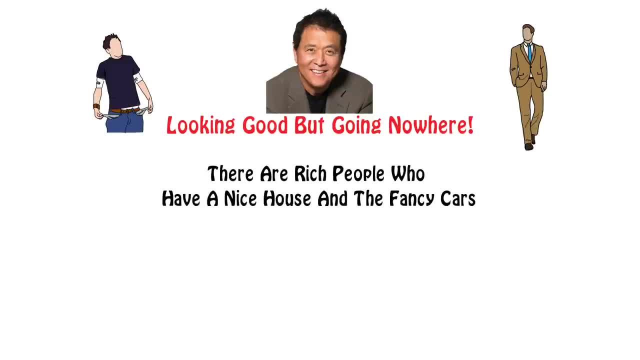 nice houses, fancy cars and all of that luxury stuff. And yes, it's true, But the main difference here is that poor people use their own money or go in debt to buy their luxuries. The rich have their assets. buy luxuries for them. 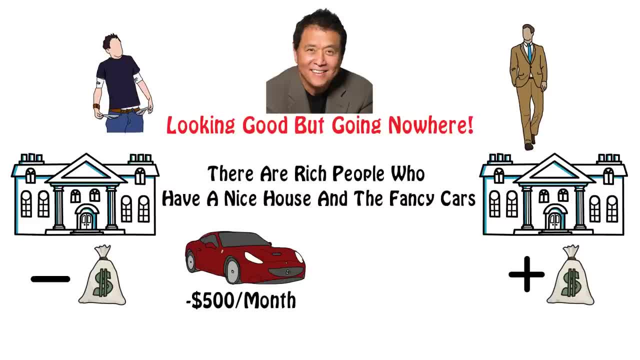 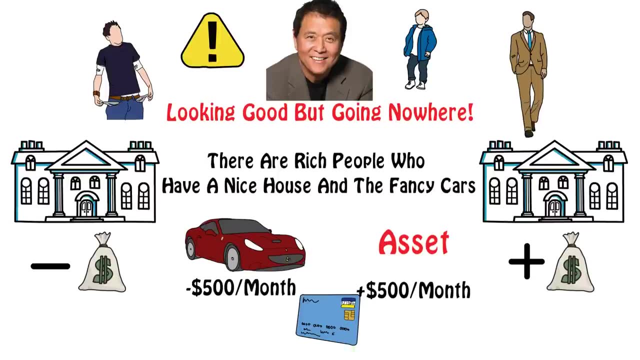 If you want a car that costs you $500 per month, well, it's time to build another asset that generates you $500 or more per month. This way, your bank account is unaffected when you buy this liability. That is another crucial element that many rich parents teach their kids. 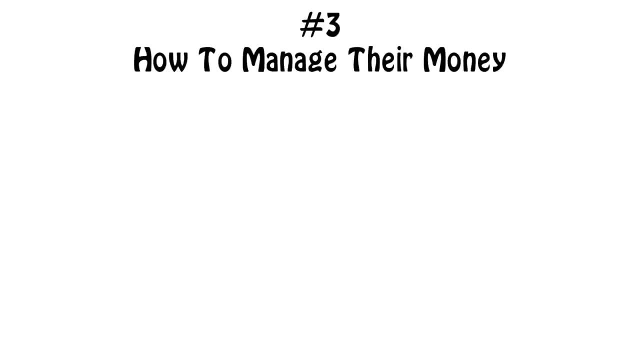 Number three: how to manage their money. A very good way many wealthy parents teach their kids about money is by letting them into their planning and managing of their household expenses. Many of these parents include their kids when they go over their financial statements and plan their budgets. 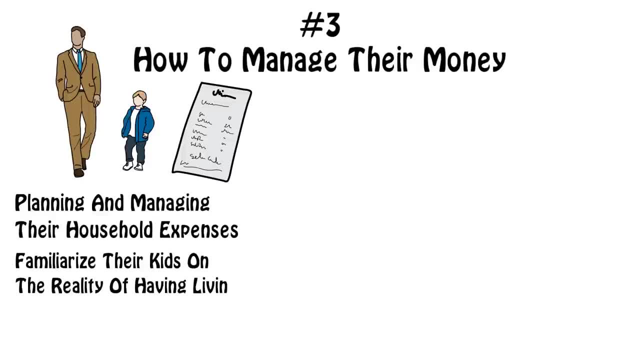 They often familiarize their kids on the reality of having living expenses. This gives their children the experience of managing money from an early age, which can help when they grow older and they have to manage their own money. This is a big contrast to many parents with a poor mentality. 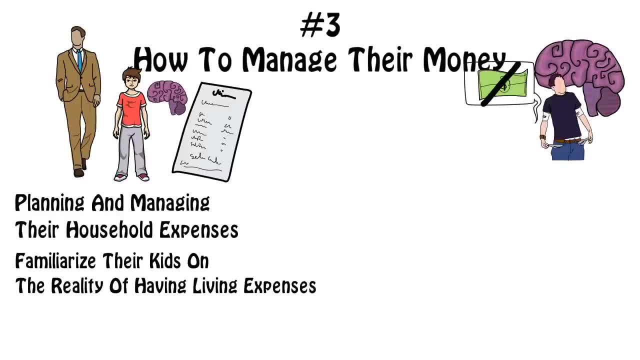 The majority of parents rarely talk about money, especially their own income. They typically plan their monthly budgets without their kids- if they even plan at all- and often associate a negative attitude when planning their monthly expense budgets. Oftentimes parents argue and express negative feelings about planning their monthly budgets. 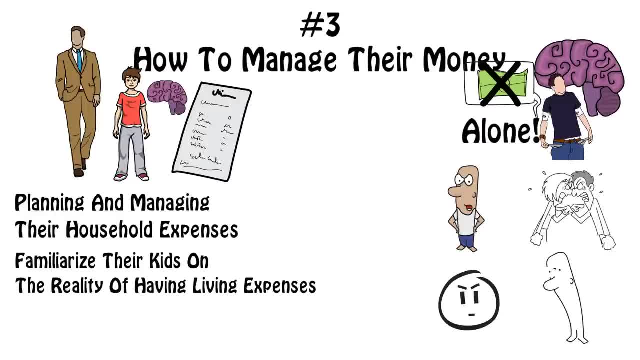 causing their kids to take on similar planning patterns, which translate to similar behaviors later in life. Rich parents know that living expenses are a reality of the modern life and focus on associating good emotions on their living expenses. As odd as that might sound, many people are grateful for those living expenses because 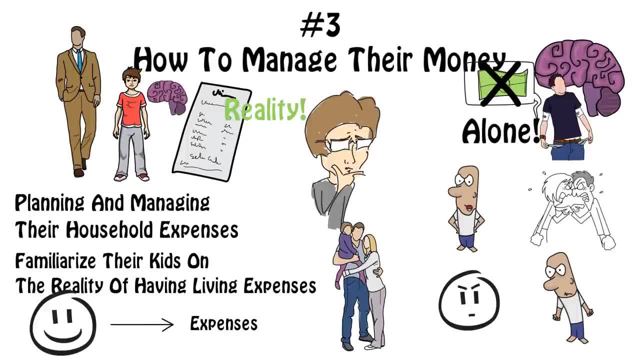 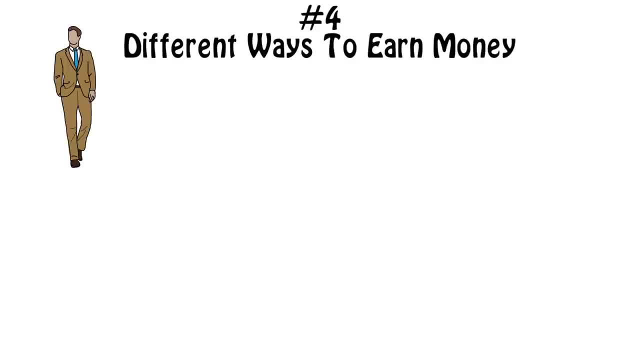 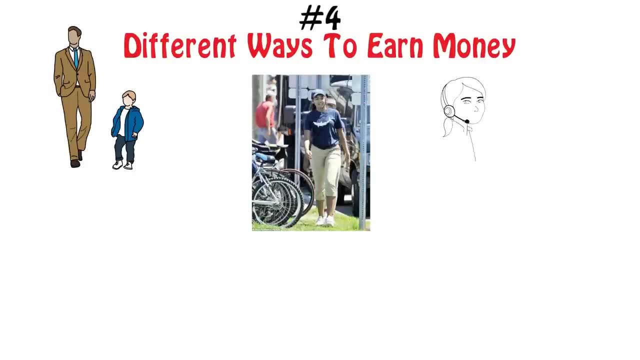 it provides them with a roof over their heads and the ability to live comfortably. 4. The Different Ways of Earning Money. One thing that I've noticed many wealthy parents teach their kids is the different ways to earn money. Did you know that the daughter of former President Barack Obama had a normal customer service? 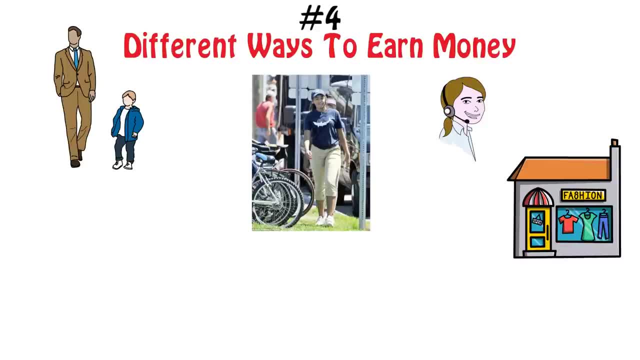 job. Many other wealthy people have their kids get a normal job. There are a few reasons for this, but one of them is to be able to have them experience the different ways money is earned and teach them how each of them work. For example, one of them is exchanging time for money, whether that is working on a job. 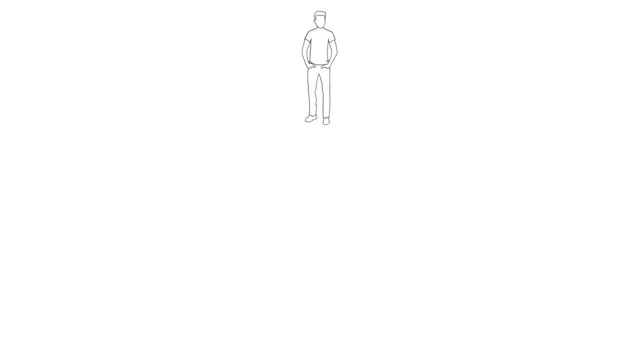 on a job or freelancing. The second is to build systems that generate you money or having money work for you, Like building a business and leveraging the time of other people as employees, leveraging online systems that provide automation, or using money to buy assets that generate income. 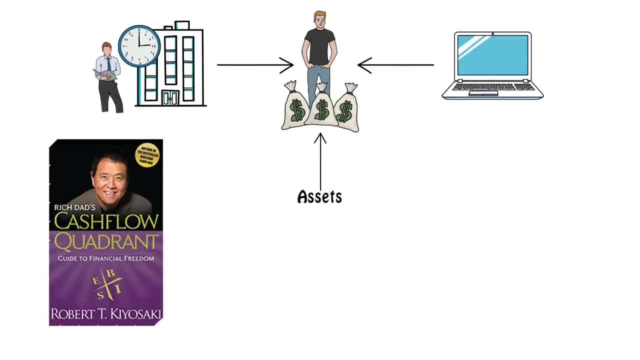 for you, Which is illustrated in the book Cashflow Quadrant by Robert Kiyosaki. The rich focus on understanding and teaching these principles to give their kids the freedom to not be stuck in one way of making money. The rich focus on understanding and teaching these principles to give their kids the freedom. 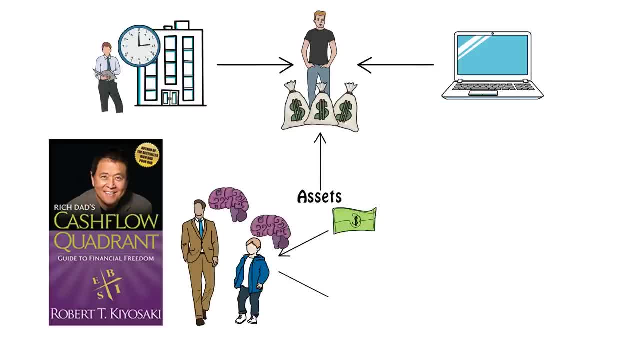 to not be stuck in only one way of making money, But give them the ability to learn the other ways money is made. On the other hand, most poor parents only know one way of making money, which is typically exchanging time for money, and, sadly, is the only thing they teach their kids, and they 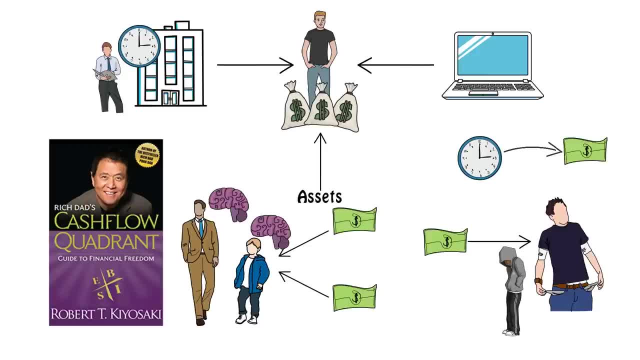 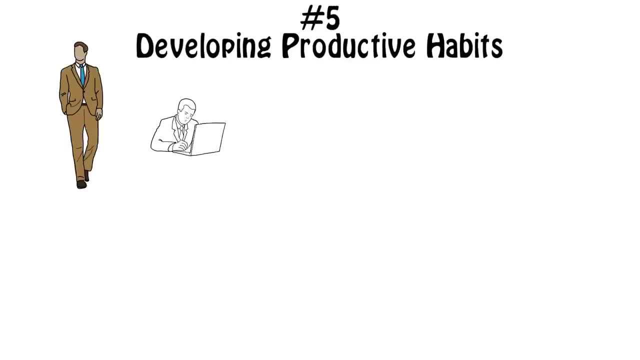 eventually grow up only knowing one way to make money, which limits their true earning potential. Number 5. Developing productive habits. The rich know that it is not what you do that makes you wealthy, but what you do consistently. If the wealthy parents are self-made, they know that in order to make money they need 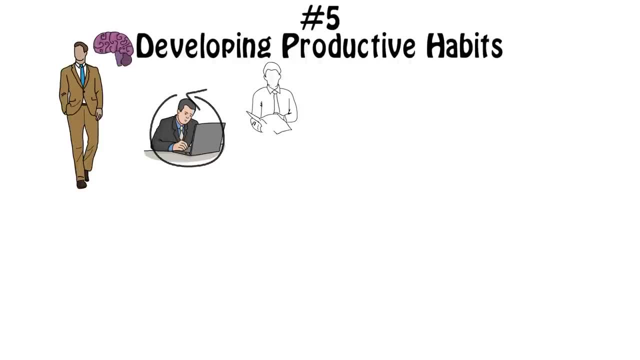 to work and carry out their plans on a consistent basis. It's not just about taking action once or working hard once, but doing it over a prolonged period of time, And the best way to do that is by building habits, things that you come to do naturally. 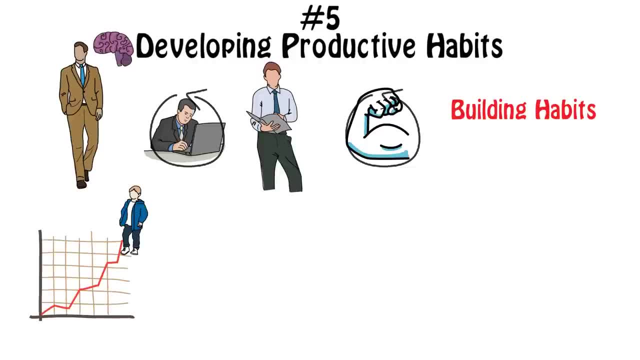 So many wealthy parents focus on developing productive habits on their children so they can attract wealth themselves more naturally in the future. This can be as simple as starting their day with a set of accomplishments, or to always look at how they can bring value to others. 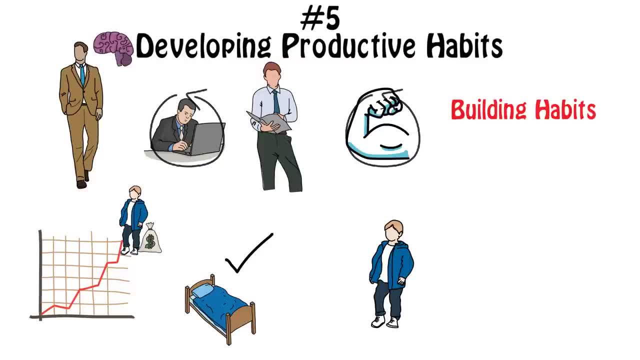 Not only that, but many wealthy parents teach their kids how to build their own habits. Learning how to build habits is one of the best skills anyone can have. Understanding the psychology behind modifying your own habits can be extremely powerful for a child's long-term success. 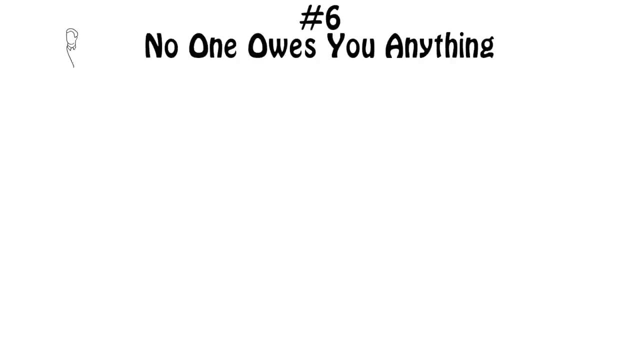 Number 6. No one owes you anything. Self-made millionaires and those who got wealthy with their own work know how much it takes to create wealth for themselves. Number 6. No one owes you anything. They know that they will only get what they fight for, and no one owes them anything. 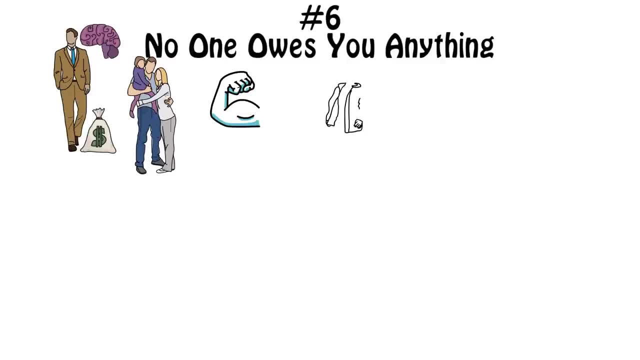 This is especially important for rich people because in many occasions their kids grow up in a wealthy environment where they can feel like they deserve to have a piece of their parents' wealth. They understand that this sense of entitlement can be a huge disservice to their kids in 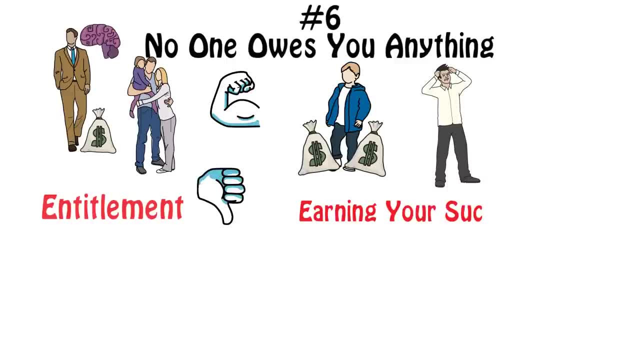 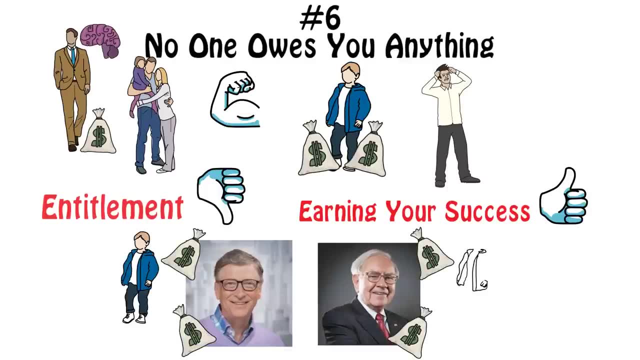 the future and teaching a concept of earning your success becomes very important to them. Bill Gates and Warren Buffet, two of the richest men in the world, have similar values. They will not leave their kids with their wealth and will only leave them with a miniscule. 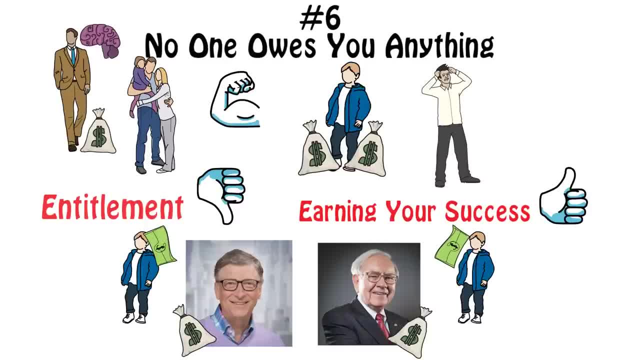 amount of inheritance. As Bill Gates said in an interview in 2011,. they have to find their own way. They try to install a sense of independence and hard work so their kids can find their own success. Number 7. Social and influence skills. 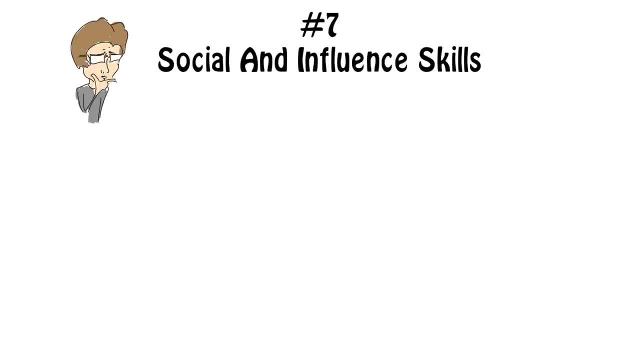 This is something that isn't talked about enough in the financial and business world, but is one of the most important. The ability to socialize and communicate with others can open up a lot of opportunities that otherwise wouldn't happen. The ability to create influence with those around you creates a sense of leadership. 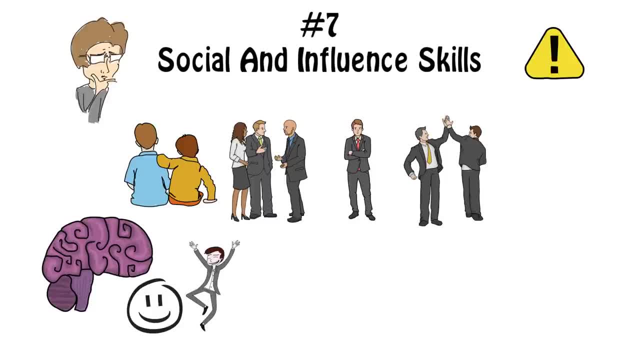 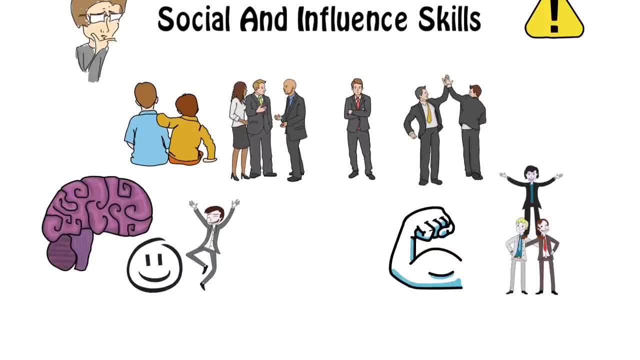 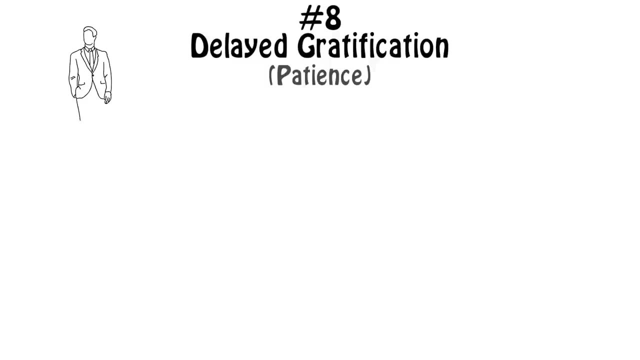 Installing that skill to understand people's emotions, motivations and behaviors early on can provide an incredible tool for the future, setting kids up to be strong and influential leaders. Number 8. Delayed gratification, In other words patience. The rich understand that completing a master's degree in financial and business is not a 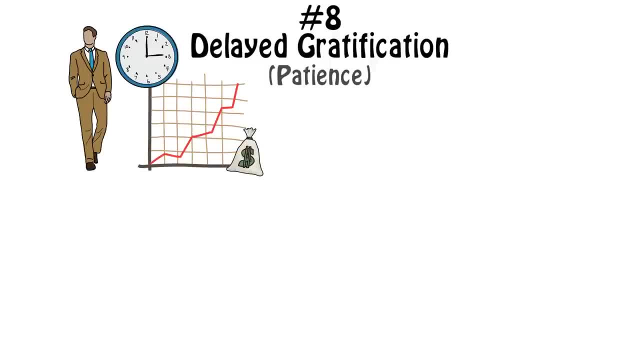 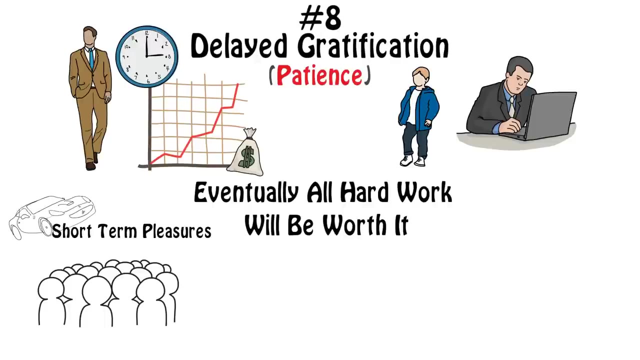 complete success. Cleaning a massive gold and building wealth takes time And they must be patient while working hard at their craft. And that is one of the skills they often teach their kids: that eventually their hard work will pay off. The majority of people prefer short term pleasures like buying the nice car or the fancy house. 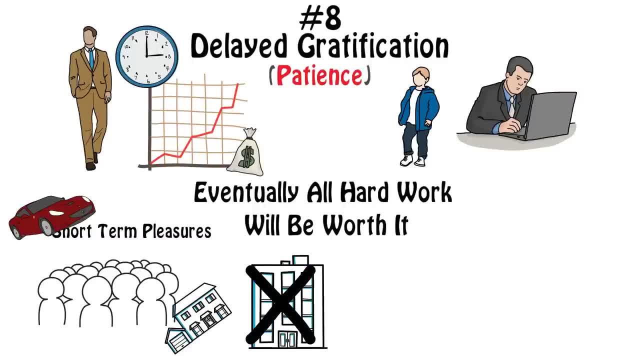 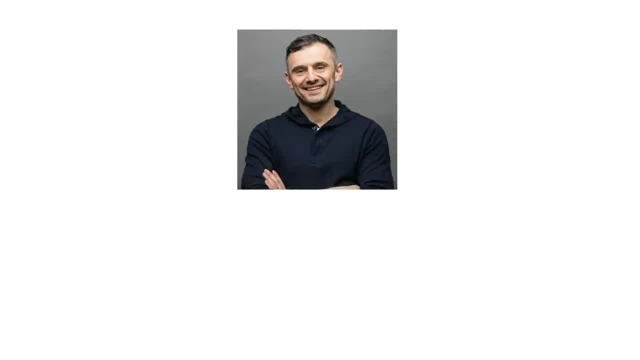 right away, or they might start a business and leave when it's not profitable in the first year, and they pass down the same behaviors to their children. I really like something that Gary Vaynerchuk says when it comes to this Number 9.. 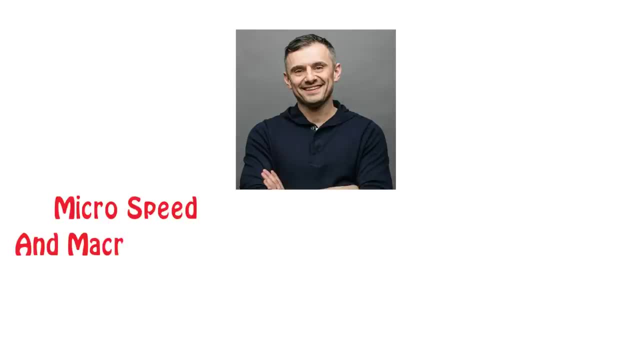 Microspeed and Macropatience, That is, to have microspeed and macropatience, meaning we must work hard consistently every day and be patient for the big picture. As he says, most people are slow on the day to day and want to be successful the next. 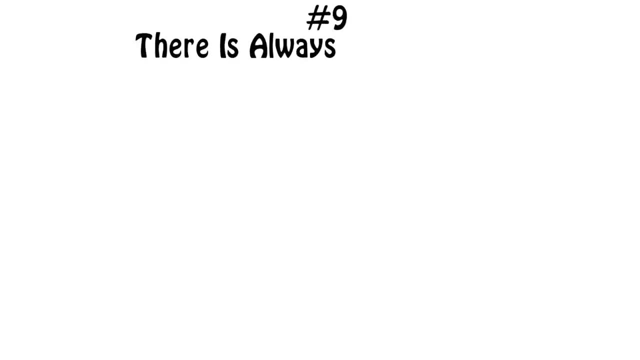 day Number 9.. There is always more money. An incredibly important mindset that the rich have is that there is always more. Most people think that there is a limited amount of money in the world, And that belief translates to their bank accounts. 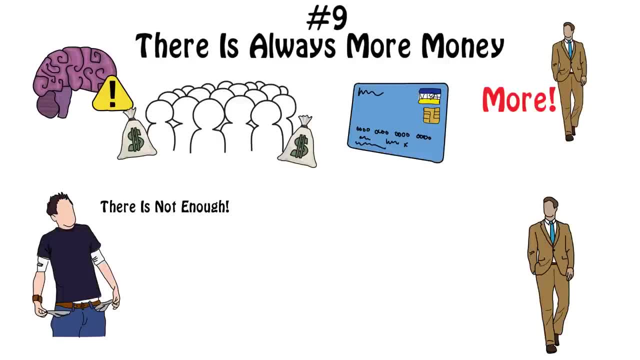 While the poor might feel like there is not enough money, the rich know that there is always more money out there, Whether it's to fund a new business or take a vacation. they know that there is a lot of money out there and their job is to get it. 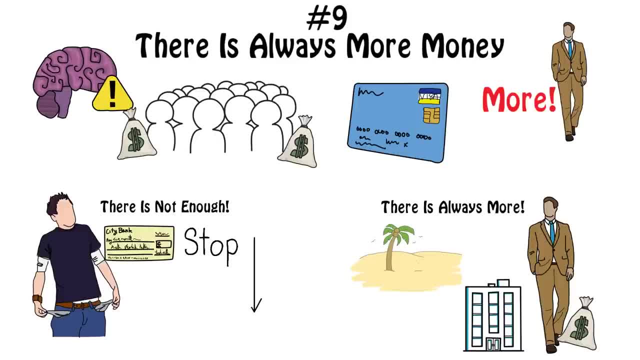 The poor think that their salary is their financial limit and they will have to live under this financial ceiling, which is a scarcity driven mindset. The rich know that there is no limit on how much they can earn and money is out there waiting for them to watch out. 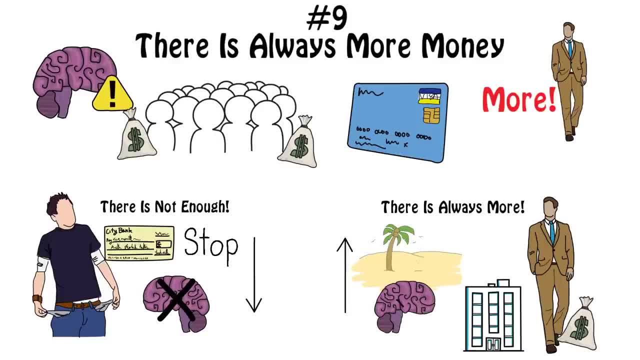 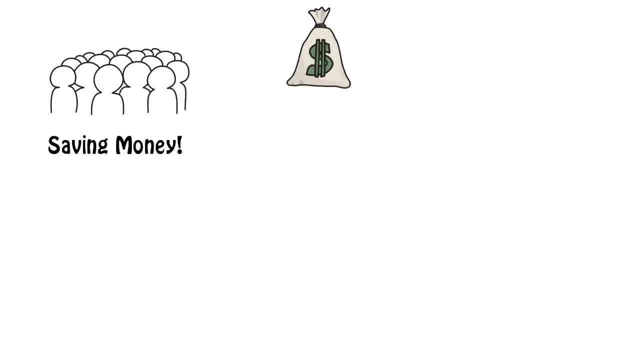 This is a simple concept that can play a major role in our financial decisions. While most people focus on saving money and reducing cost, the rich focus on increasing their income. This doesn't mean that the rich don't focus on reducing expenses, but they invest. 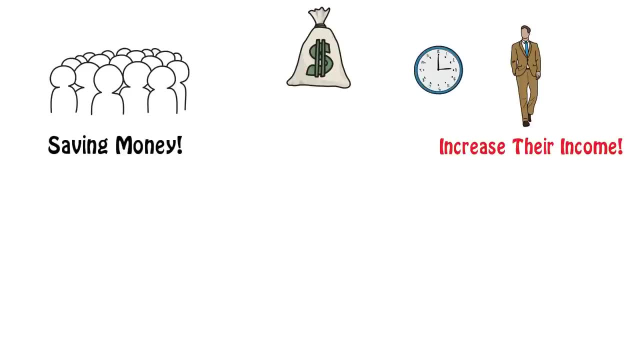 more time and energy in increasing their cash flow over reducing a few small expenses. As a business owner, having a scarce mindset can limit the entrepreneur's earning potential. There are many entrepreneurs who don't charge what they earn. They don't have enough money. 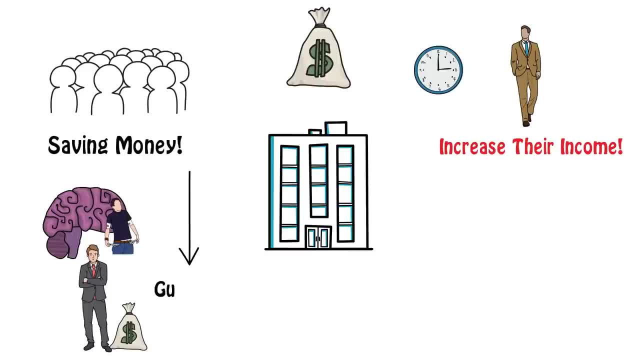 They don't know what they deserve for their products and services simply because they feel guilty for charging money to others. They might feel like they are doing a disservice to their clients by taking their money, But an entrepreneur with an abundant mindset knows that anyone has enough money for the. 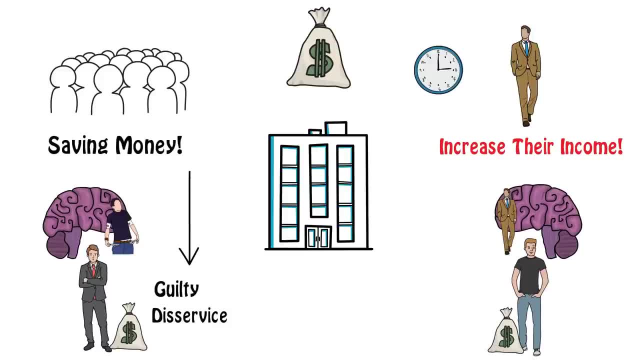 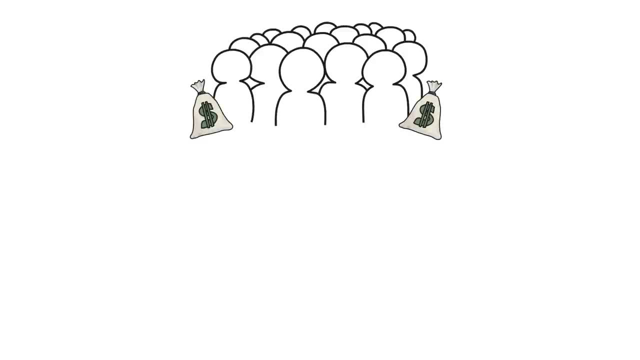 things they really want. And if a potential customer wants their product, who are they to deny it? If you take a look at society, people always have money for the things they really want. If they want to go on a nice vacation, they spend months saving for it. 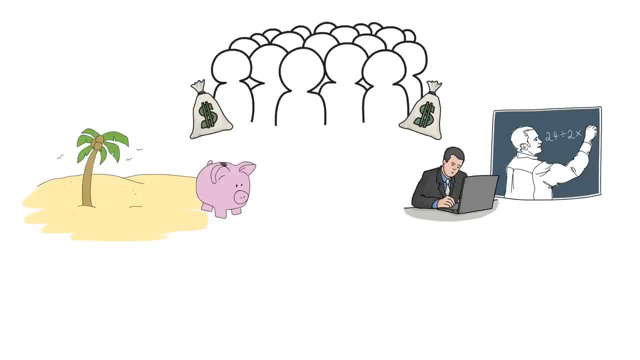 If they want to invest in their business, they spend months saving for it. If they want to invest in their education, they will work an extra shift to buy that course. If they want to begin investing, they will work hard and save to start investing. 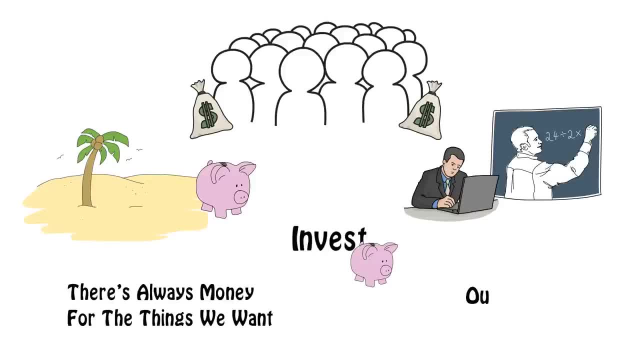 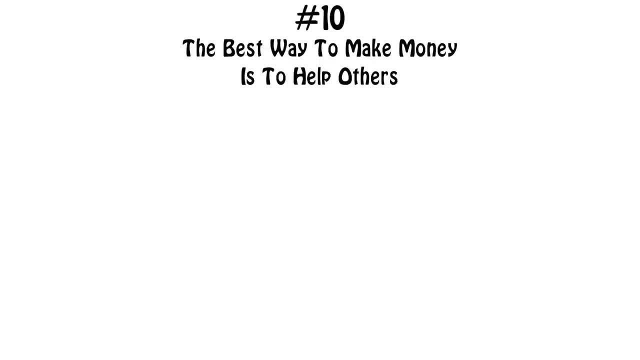 There is always more money for the things we want. Our job is to go and get it 10.. The best way to make money is to help others. An important lesson that the rich teach their kids is that the most powerful way to make money is to solve other people's problems. 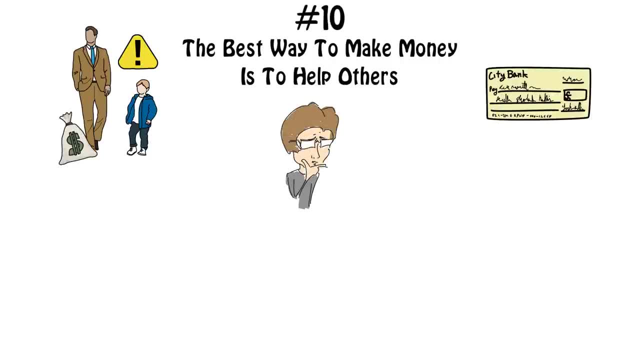 And the bigger the problem, the bigger the problem. And the bigger the problem, the bigger the problem The paycheck. It is no secret that the most successful people in the world have solved, or at least aid in solving, big problems in the world. 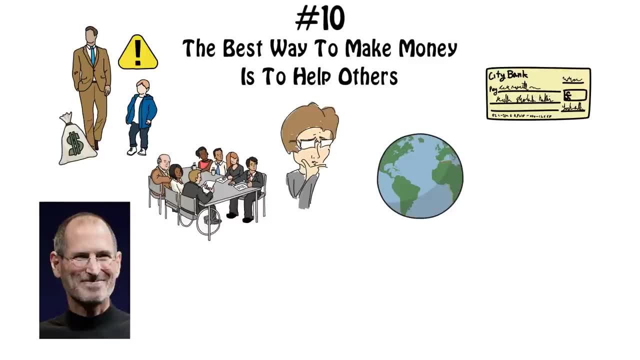 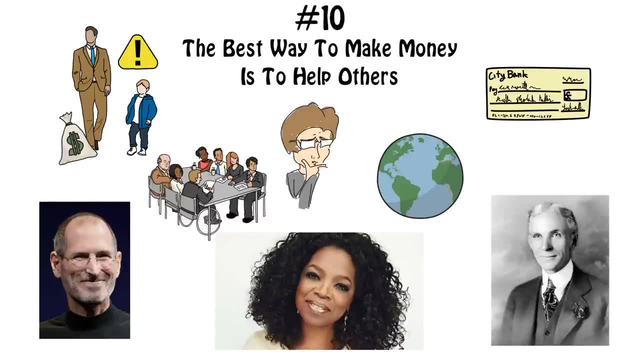 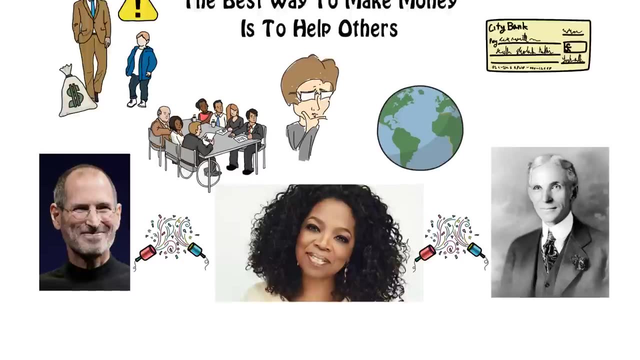 From Steve Jobs for revolutioning the technology, music and communication industry, to Henry Ford for transforming the personal transportation industry, to Oprah Winfrey for making a global impact in the self-development world. All made a huge impact in helping others solve a problem. 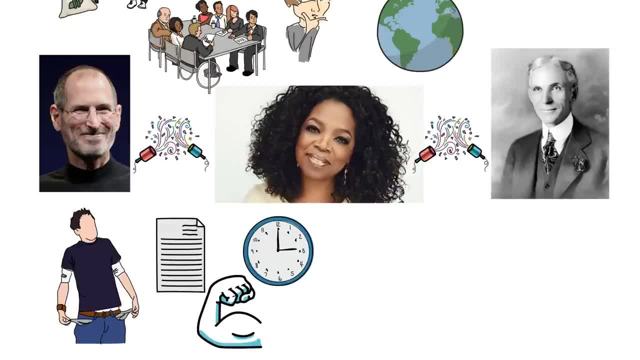 Most poor people focus on getting paid based on tasks, efforts and time, While the rich focus on providing results and solving problems. Providing value is the rich person's game, and they get paid based on the amount of value they provide: 11.. 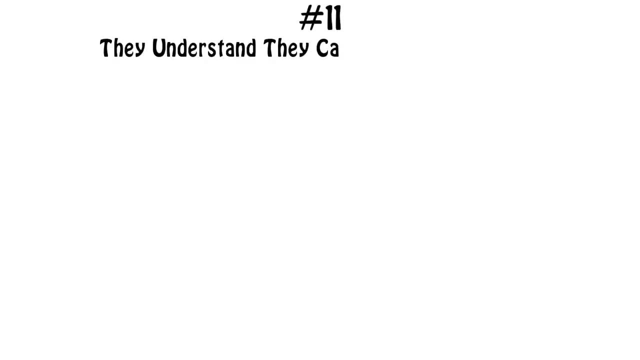 They understand they don't know everything. Something that the majority of people don't know is that rich and successful people get together in groups called masterminds. They know that it is impossible for them to know everything, so they spend time with others who know things they don't.